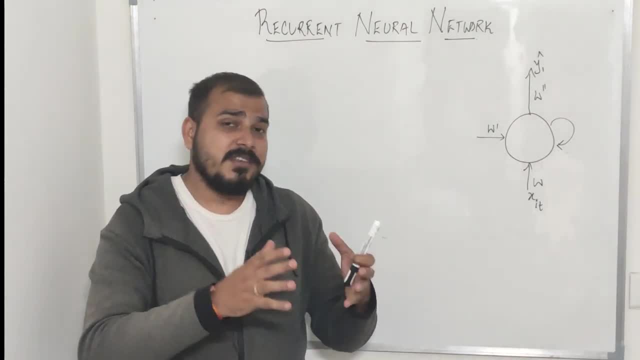 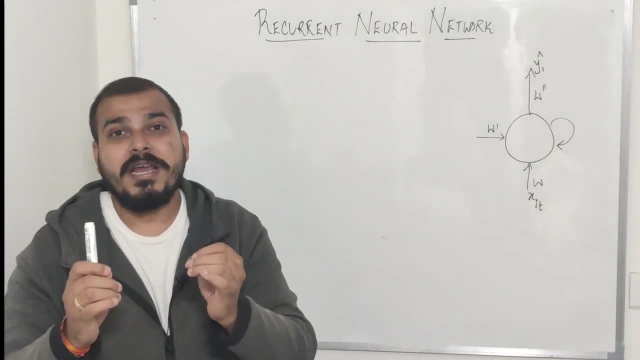 I can actually be implementing, using a recurrent neural network, Time series data, sales forecast, stock forecasting. you know, stock forecasting. many more things can be done with a very good accuracy with the help of recurrent neural network. Okay, so let us go ahead and try to. 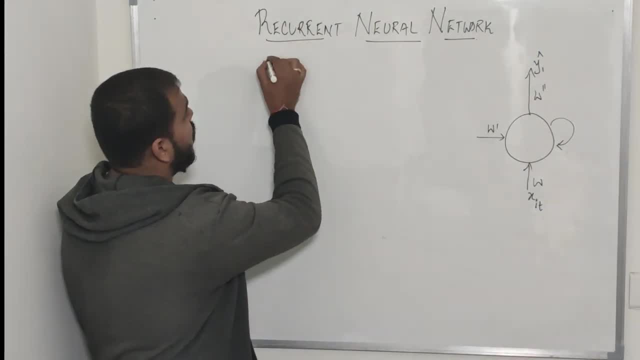 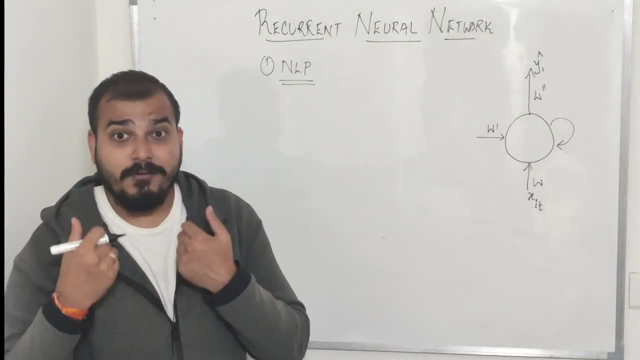 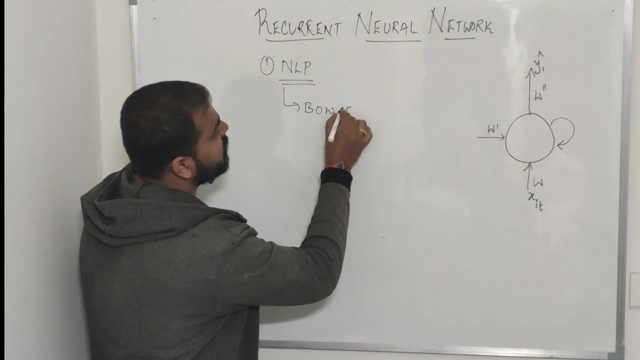 understand why exactly RNN. Now, guys, if I take an example of NLP, that is, natural language processing, and till now, if you know, machine learning. in machine learning- I have already uploaded videos regarding NLP. in machine learning, We use techniques like bag of words, right? we use? 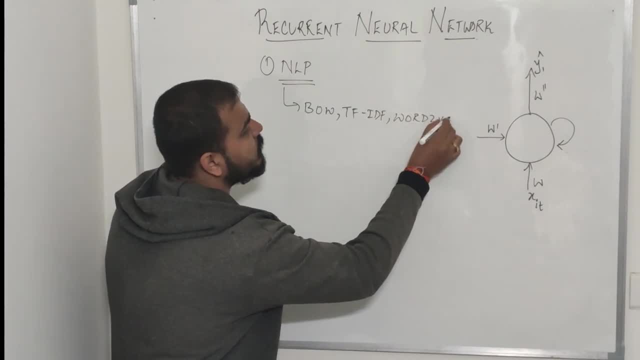 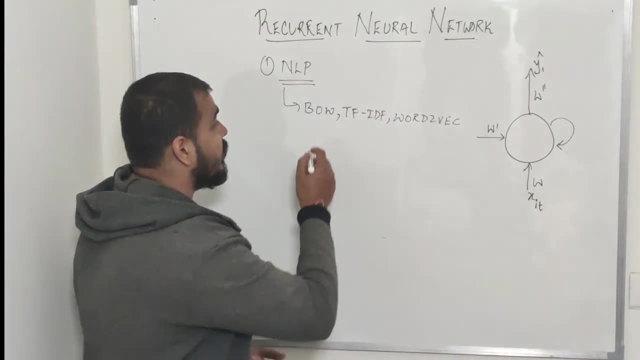 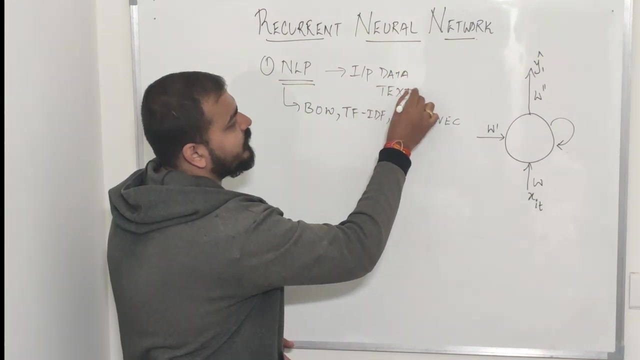 word2vec and various other techniques. okay, In word2vec we have libraries like gensim and all Now in this particular libraries, guys understand that. suppose my in my NLP, my input data is basically my text data, right, So it is text data. suppose I am doing a spam classifier. 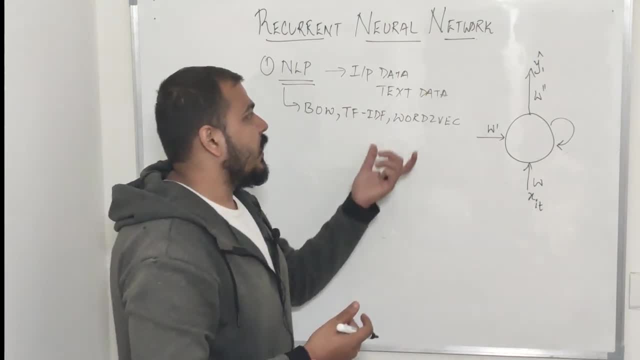 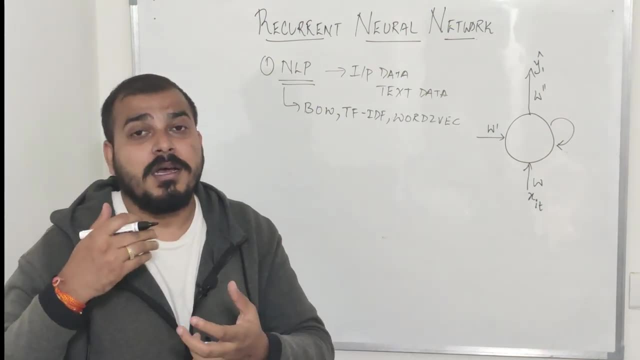 Now, based on this particular text, it should be able to derive, you know, whether this is a spam or whether that is a ham right, Whether this is a spam email or is not a spam email, right like that. So if I am using the text pre-processing techniques, some, 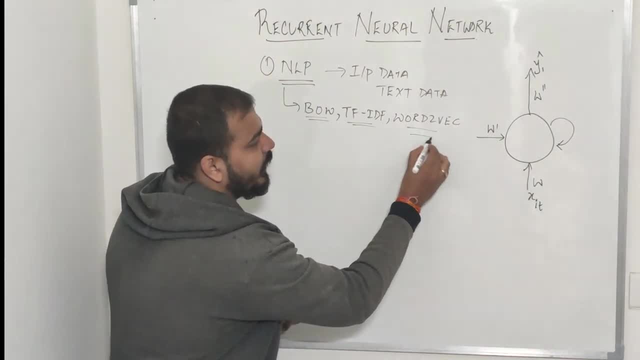 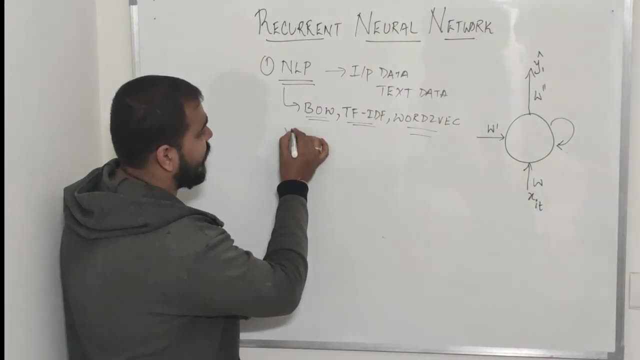 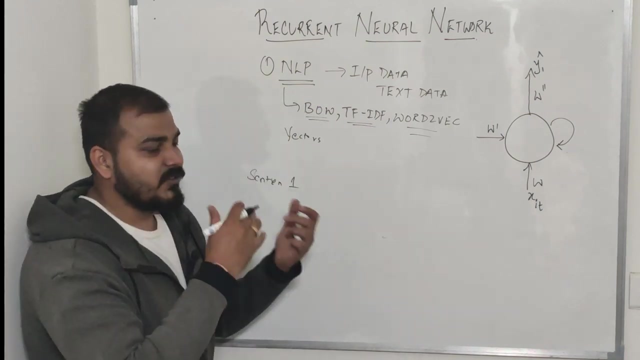 of the techniques are bag of words. we have tf, idf and we have word2vec. What are these techniques doing? we, it is basically converting this text data into vectors. okay, a very important thing like vectors, And I have told you- suppose this is my sentence one. okay, and guys, I am just giving an. 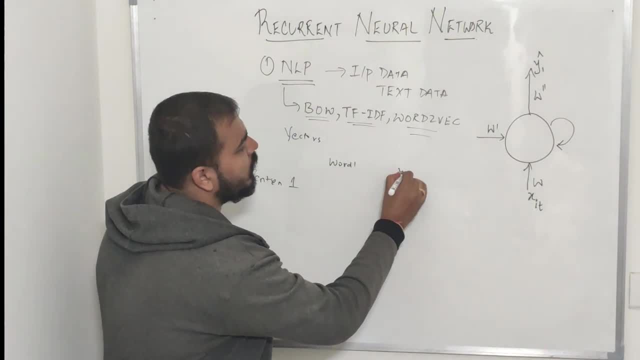 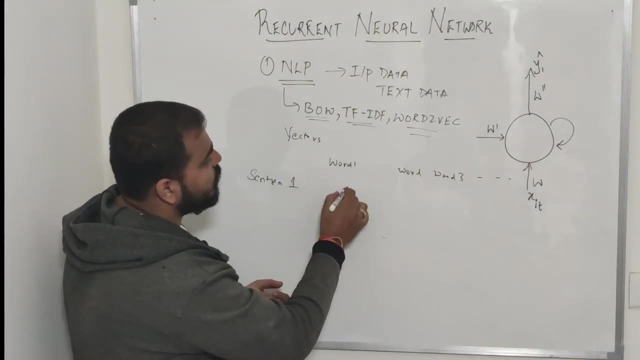 example over here. So suppose this is my word, one word, two word, three word, four, like this. some words are there, So vectors are nothing, but based on this sentence, this words will be given some values like 1, 0s, 1s, 0s, And if I consider tf, idf, it will be given. 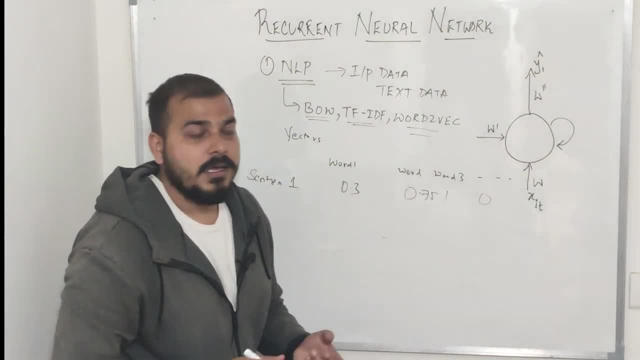 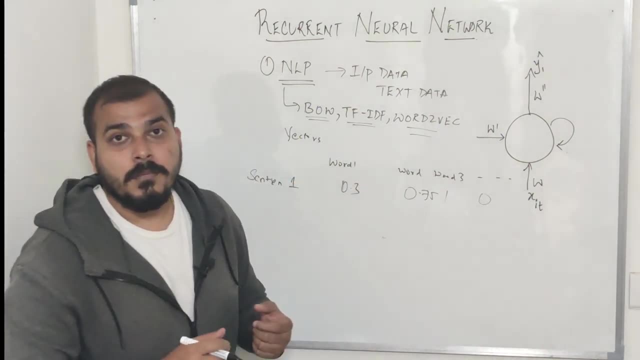 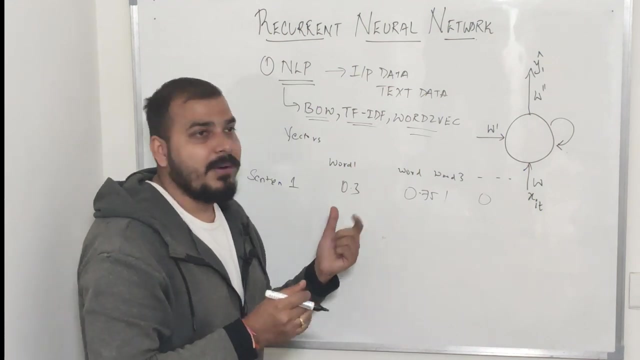 in form of fractions like 0.3.. 0.75, like that. okay, So these all are vectors and we can, we can send these vectors, you know, and so once this text data is actually converted into vectors, then we can apply a machine learning algorithm and the most suitable algorithm that we apply something. 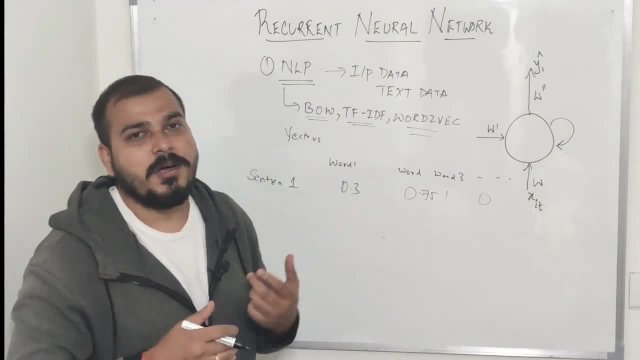 like NAVE bias And the most suitable algorithm that we apply is something like NAVE bias And we'll try to find out whether this particular sentence is positive or negative. okay, if i'm suggesting for a reviews, if i'm suggesting from spam or ham, something like that, but understand. 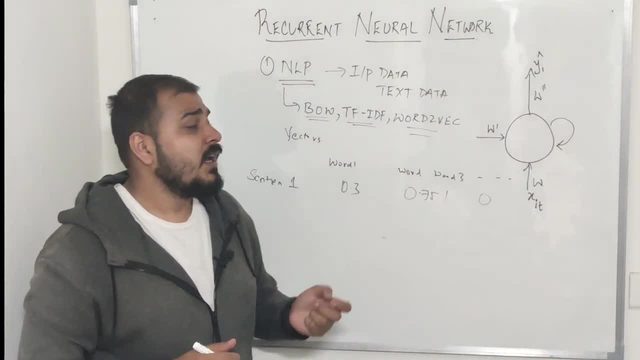 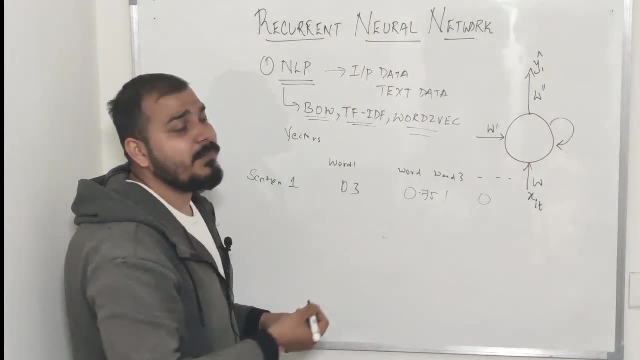 one very important thing from this particular text: pre-processing techniques, that is, bag of words, tf, id of a word to back the sequence information is discarded. the sequence information? what do i mean by sequence information? suppose i say my name is krishnayak, right? oh yeah, i have some sequence, i'm. 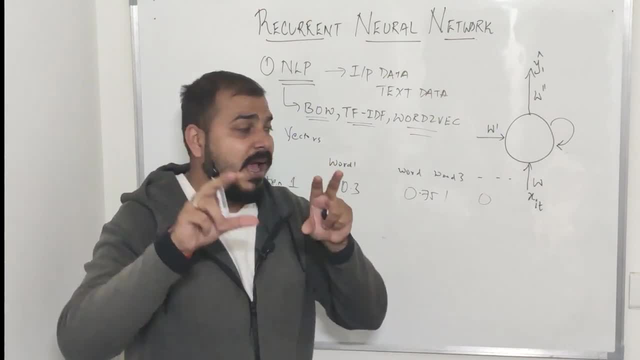 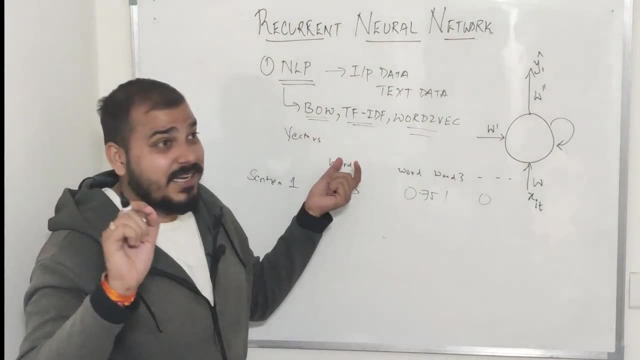 telling in some sequence, so that sentence makes some sense. you know, and that sequence over here, when we are converting this into vectors, it will get discarded, right? and please, guys, if you know about bag of words and tf, idf, if you don't know it, please go and have a look onto this, right? the. 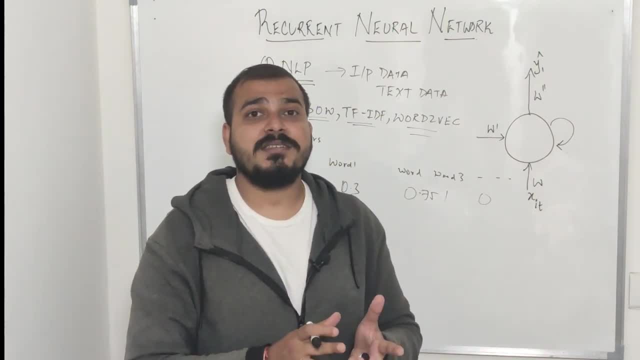 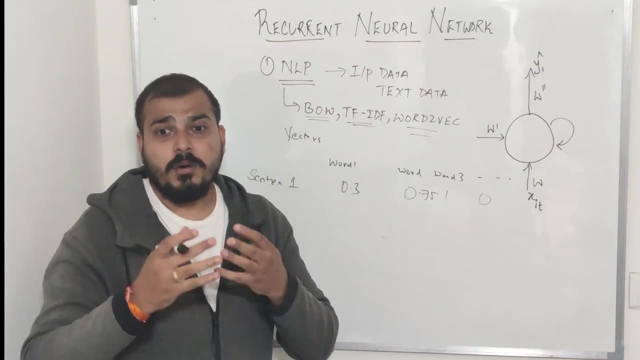 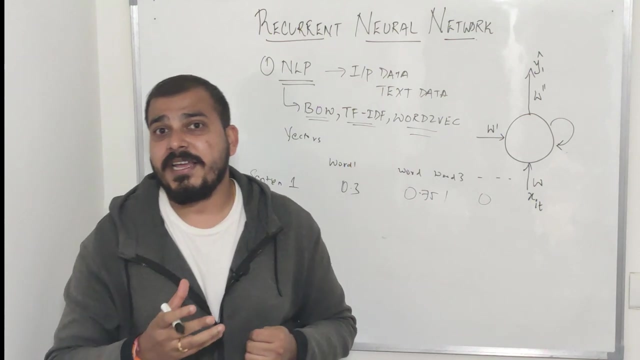 sequence information is discarded. so once the sequence information is discarded, your accuracy may actually deflect towards the lower side. you know it may go towards lower side. now let me take very good examples of- uh, now you know this- this recurrent neural network where it is extensively used, suppose. if i take an example, 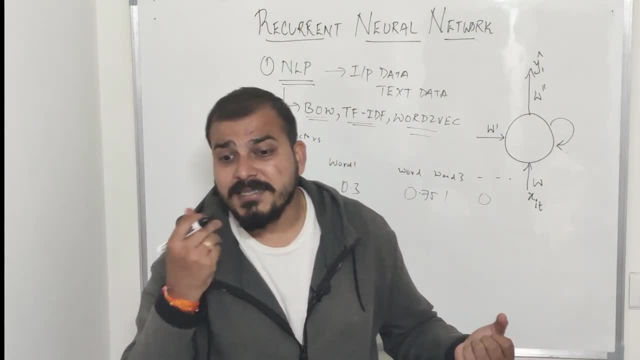 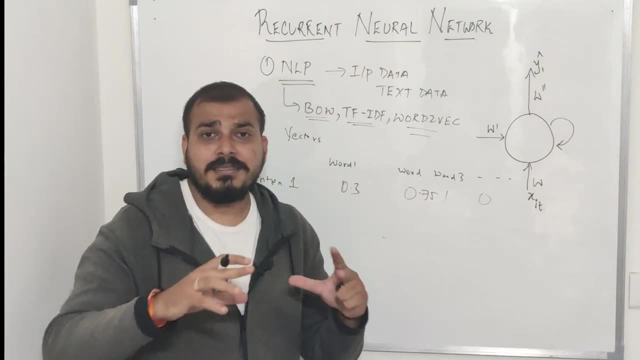 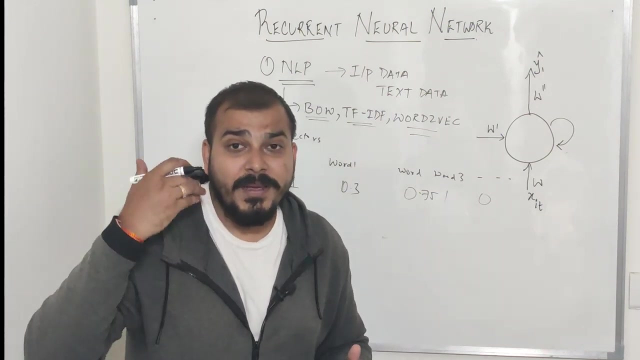 of google assistant, amazon alexa. right, if you're asking some questions, suppose you ask amazon alexa saying that what is the temperature outside, it will be telling you that particular answer in proper sentences. right, question answer applications where you, where you require such kind of answers, where you'll be able to understand right from chatbots, from from this alexa, from this. 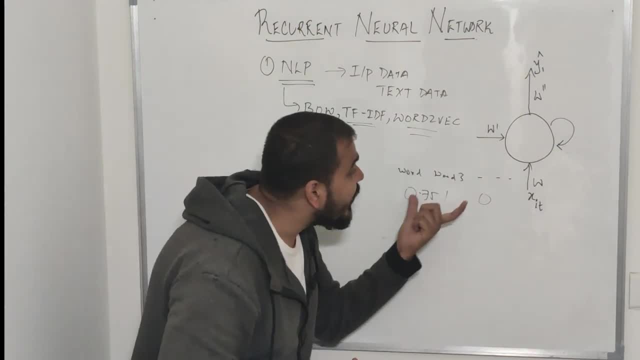 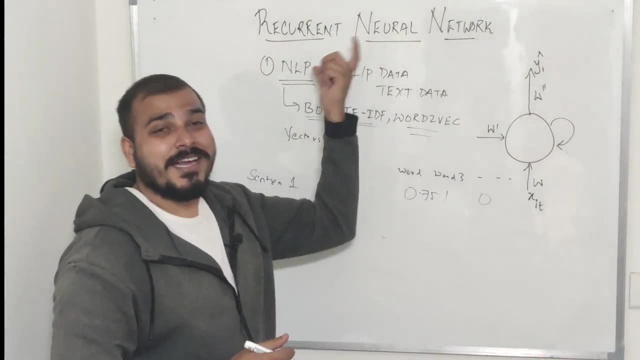 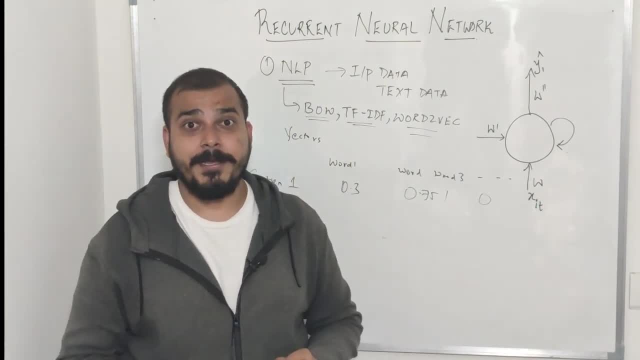 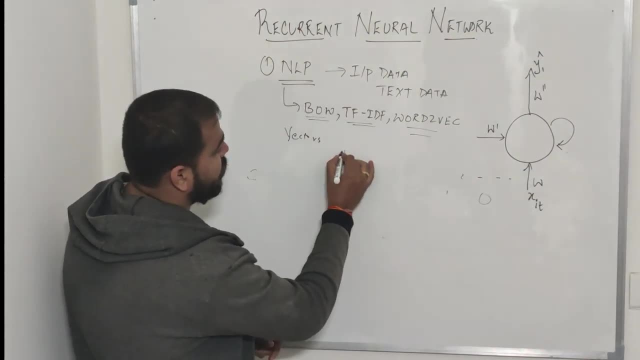 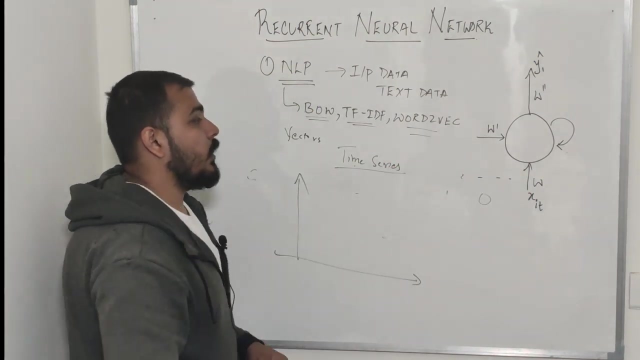 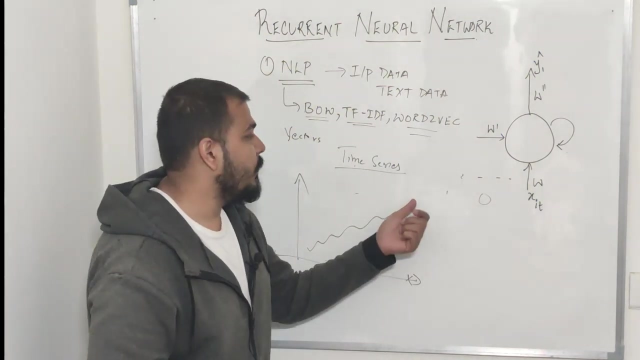 the whole maths behind recurrent neural network and they'll give you much more idea. the second type of application where it is extensively used is something called as time series. time series, let me consider an example. okay, so in time series, suppose this is my sales of a data at this particular time. i need to predict what will. 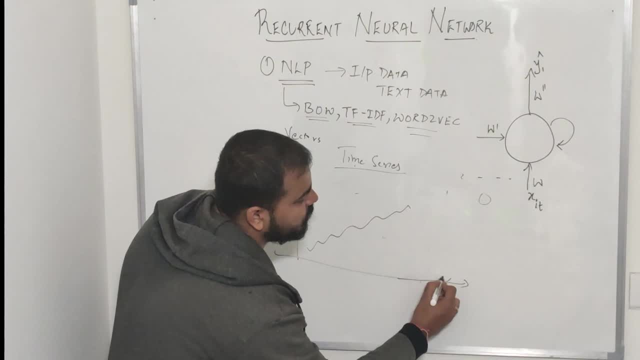 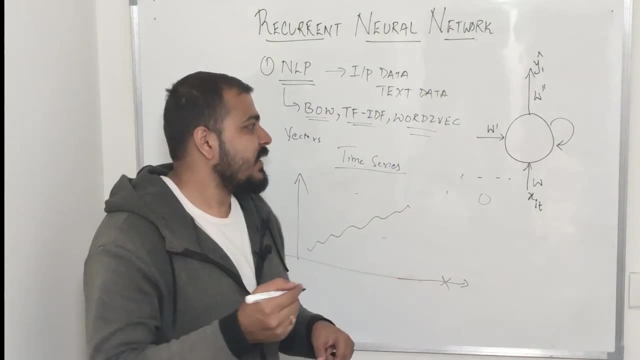 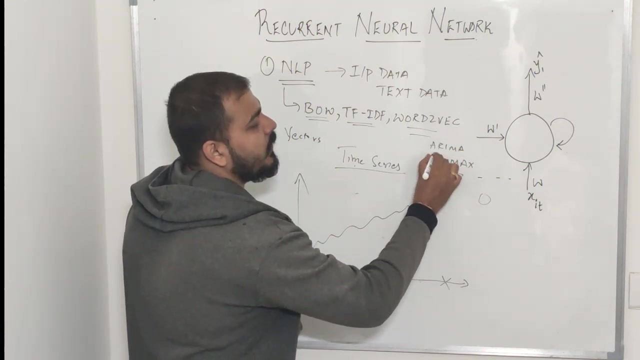 be my output, or let me just say that at this particular time, i want to predict what is the output right now. if i go in machine learning, usual financial techniques, i have something like arima- okay. i have sarimax and various other techniques. okay, and this arimax and sarimax you will be using. 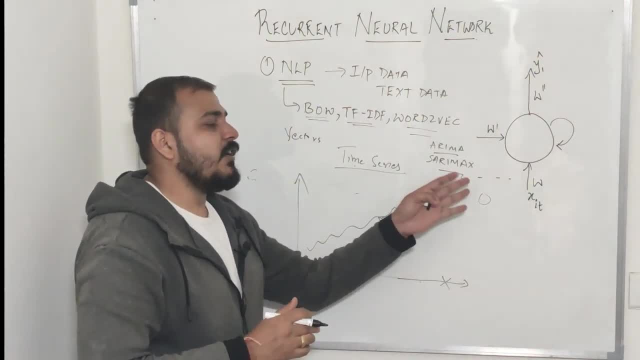 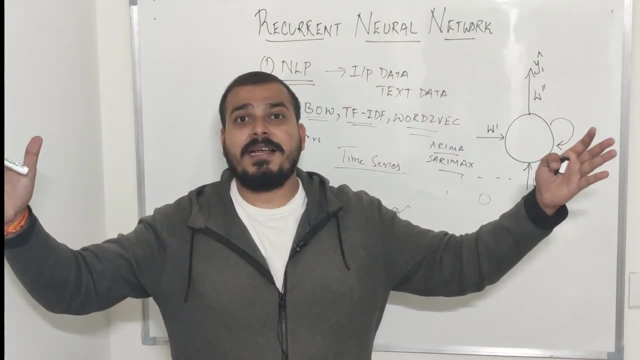 some, some windows of previous days and will try to predict the future. but in recurrent neural network- suppose it wants to predict this- it will. it will make sure that you have some timestamps that it has to consider and if i'm considering lstm, that is long short term memory again that i'll be discussing in the part. 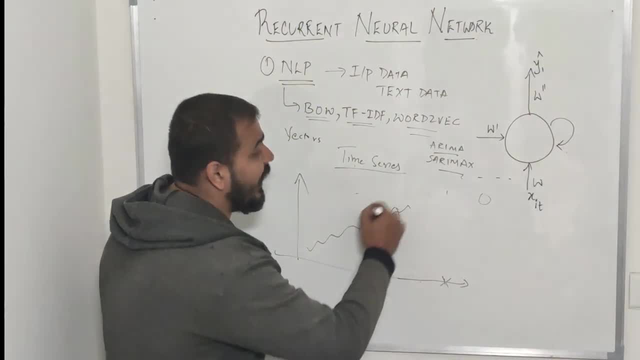 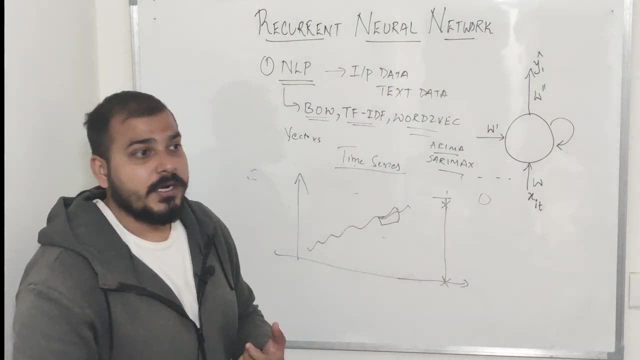 three, okay, but in this part one just understand that in this time series kind of data also, this recurrent neural network will be helpful in predicting the output. you know what, what output it will be. it will try to consider the whole time blocks, whole previous data and again there will be. 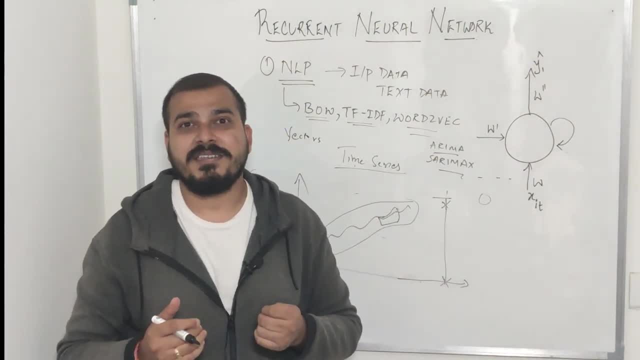 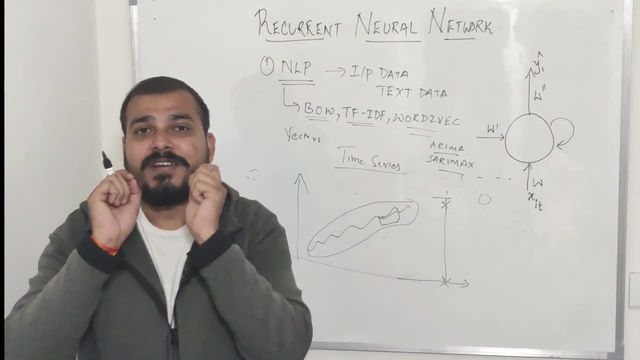 some windows block also for that, based on the lstm conditions that we basically have again right now for this kind of time series data, for this kind of nlp data, recurrent neural network is very, very good and this is this is proven to us because we have applications that are working on rnn. 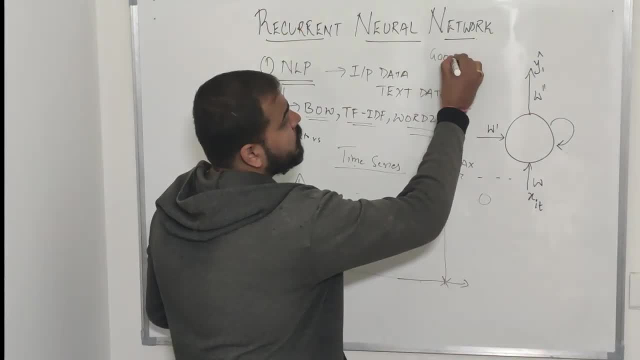 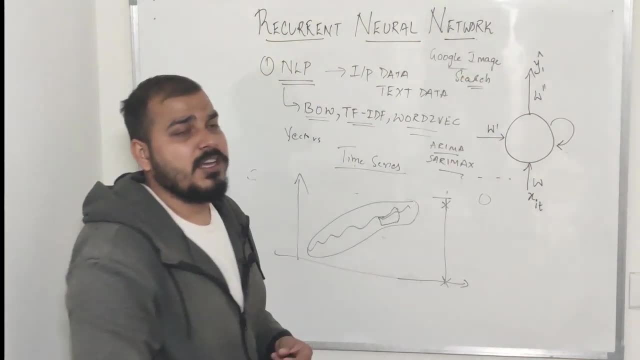 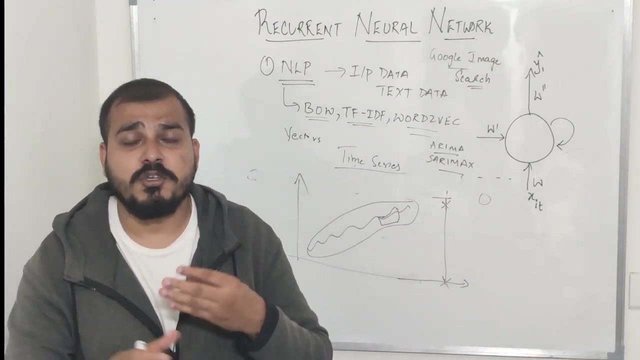 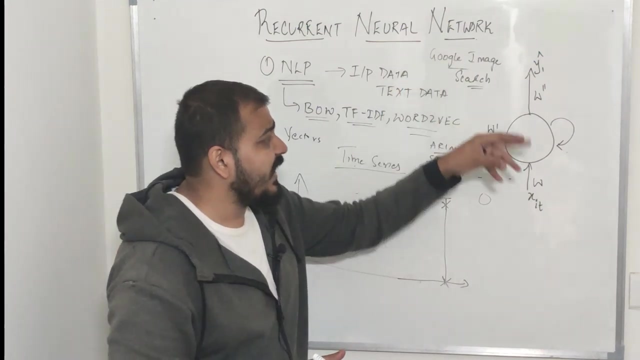 okay, some of the applications. i'll say google image search, google image search, okay. now suppose, if you are searching for something indirectly, the google image search in terms of images, right. suppose you search over there deep learning. suppose you search a neural network. suppose you search cat dog, right. so in that case what happens is that this: 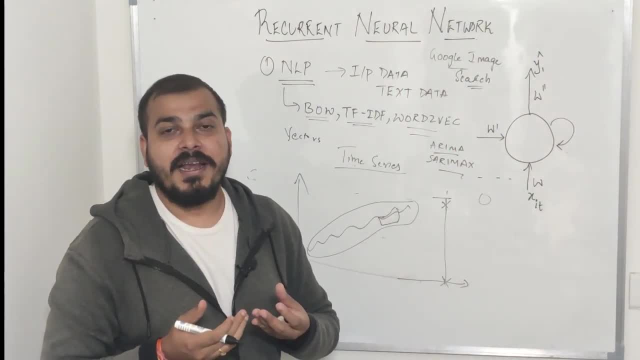 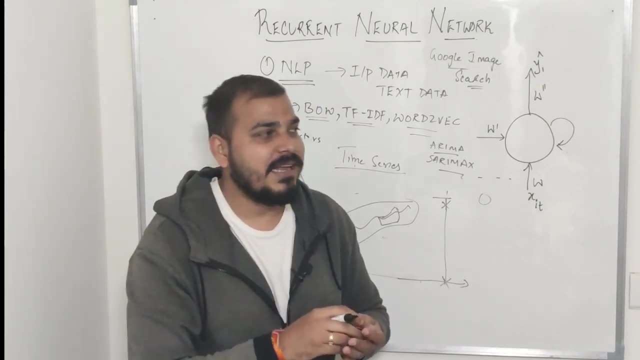 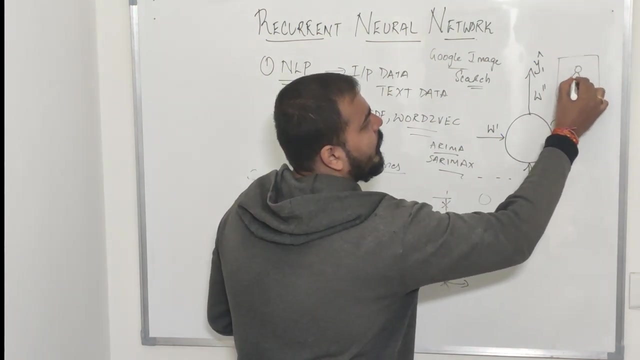 whole text. whatever you are searching, is getting converted into an image, right, and vice versa also. it happens. we usually have an application which is called as image captioning. now, image captioning: what it happens is that an image is given to you. suppose the image is like a dog is jumping a bar? 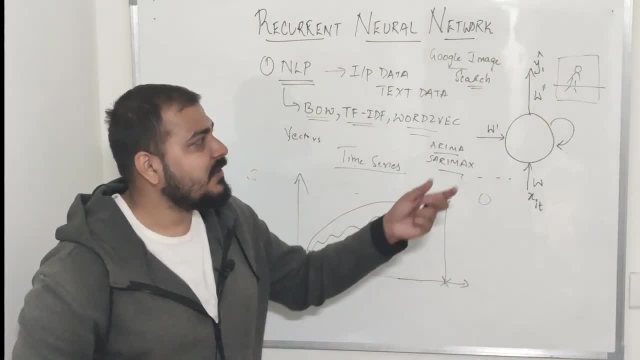 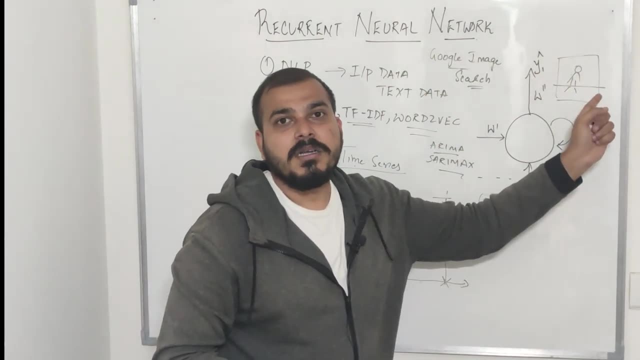 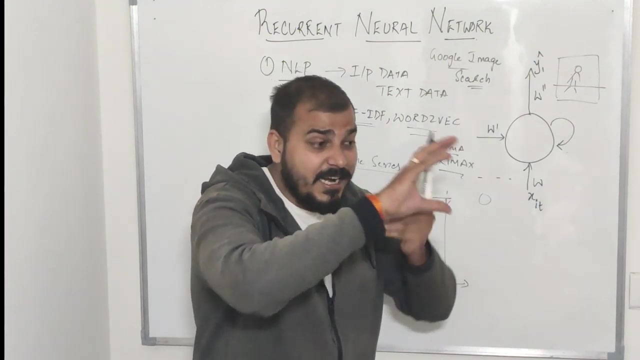 man is jumping a bar. suppose he is jumping a bar. he has this kind of images over here, so automatically, with the google captioning, with the help of recurrent neural network, will be able to convert this image, whatever it says, whatever it sees over there. sorry, suppose your man is standing over here and he's trying to jump this bar. it will try to convert that into a. 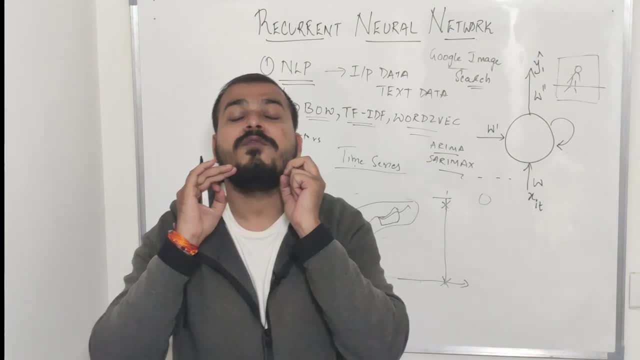 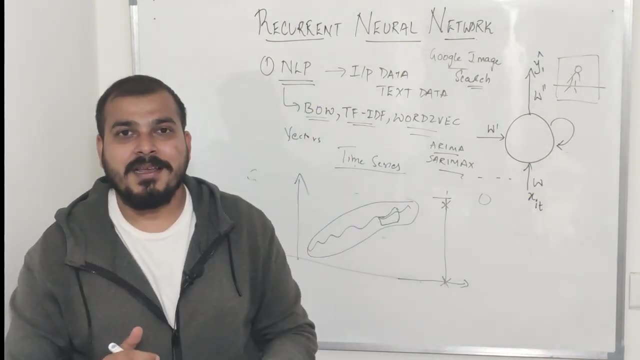 sentence and give it to you. google translator is one of the fundamental and it is again. i'll be discussing about the various types of rnn. that is something called as many to many rnn. so if you want to convert anything from english to french english to spanish, as you write on the 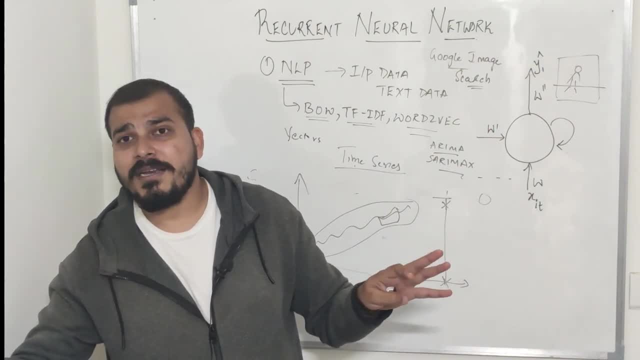 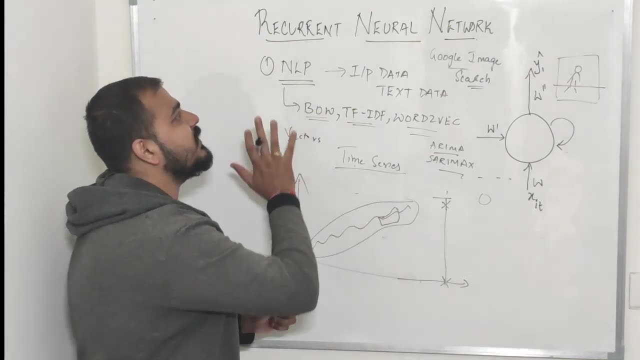 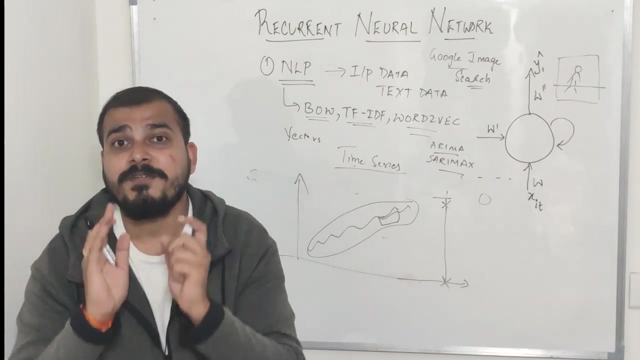 sentences automatically, the words gets converted into spanish and it makes sure that the sequence information is kept right. so it is very, very important that you understand. recurrent neural network is heavily used for sequence information of input data, and if you want to become a perfectionist in that, you need to understand this whole architecture, how it works. understand, guys. 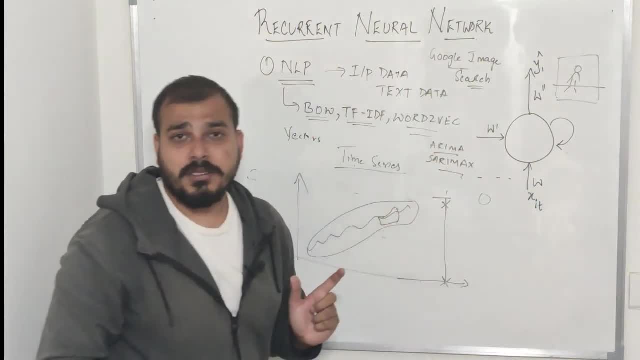 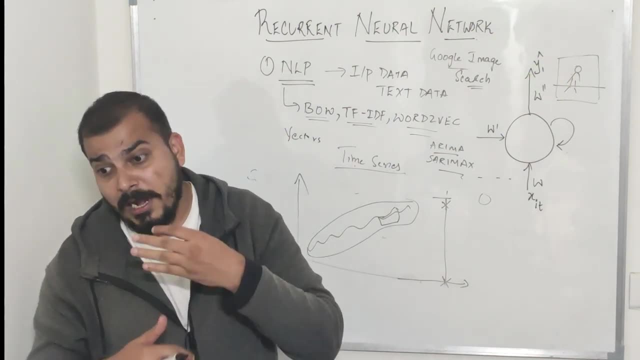 very much important. if you are able to understand the theoretical concept, then definitely you can do it with the help of coding. you know, and again i'll be telling you how i should be showing you the practical part as we go ahead. but just understand some of the applications that i. 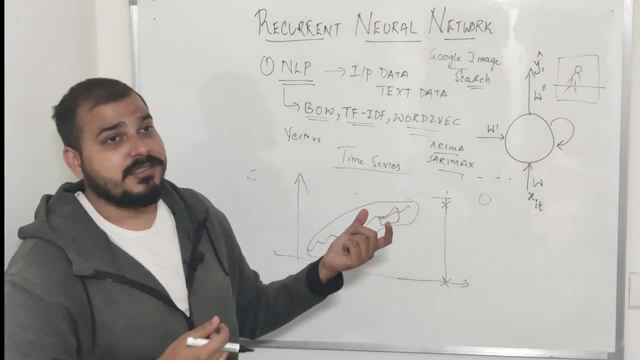 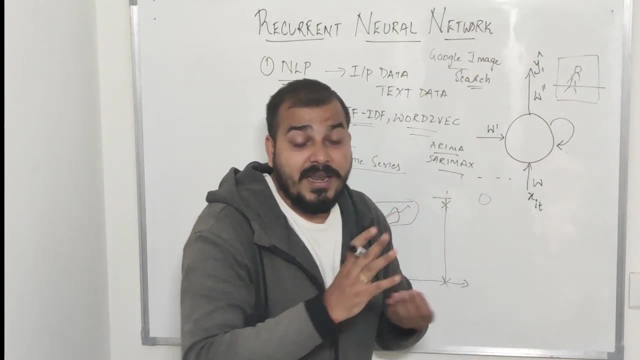 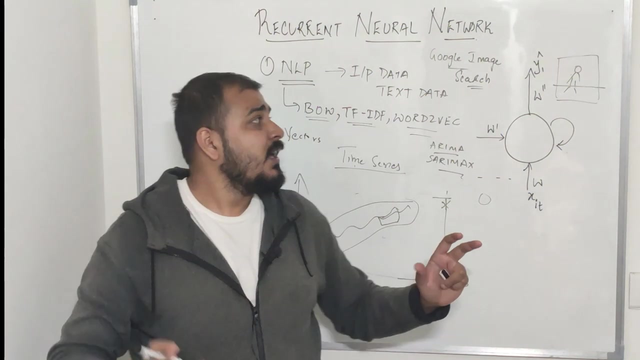 have actually done is, or told you in this particular session, is about google image search, image captioning, google translator. uh, we have nlp where i want to convert when i want to see whether a restaurant review is positive or negative. it's just a question of understanding the analysis and let us do what you are doing. 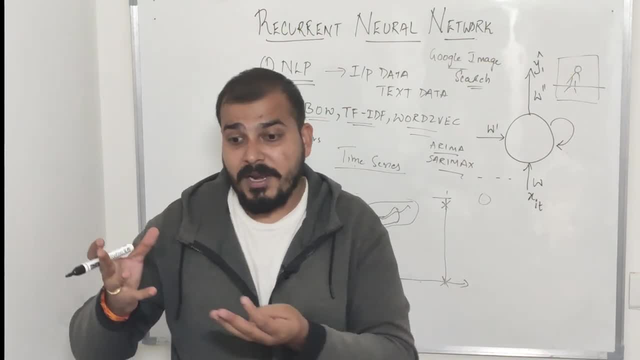 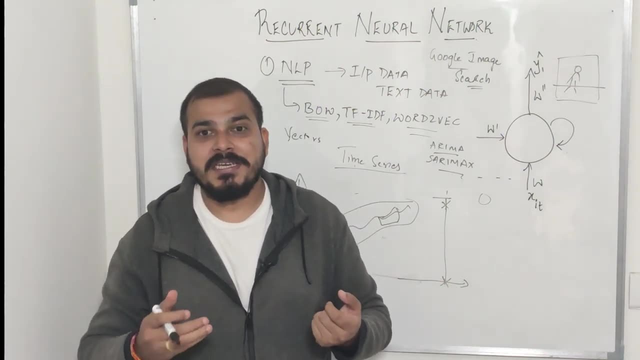 okay, so you've got your google assets in that example right under the link. so we are going to go to google and we are going to call it the data library. so here, we are going to call it the data library and we are going to tell you that. 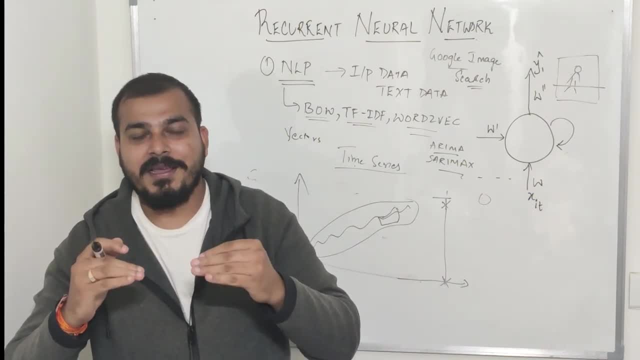 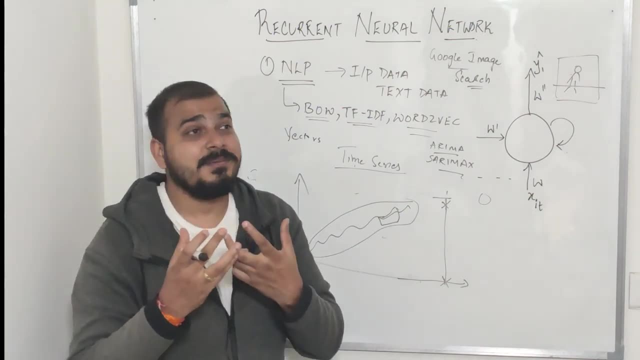 now just to see if anybody uses that data library and you are doing anything. you don't use that data. say, hey, you are intelligent man, so this, this is a kind of sarcasm. you know so that sarcasm also. people are trying to research in this. many companies are. 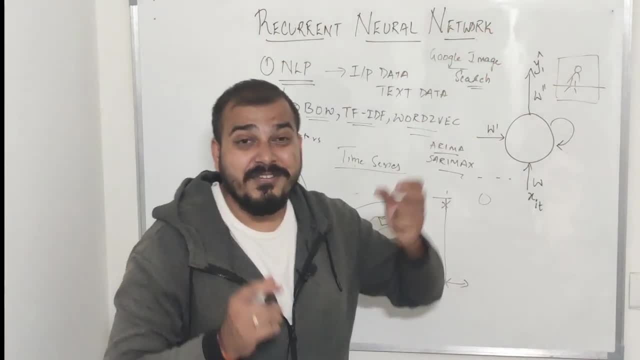 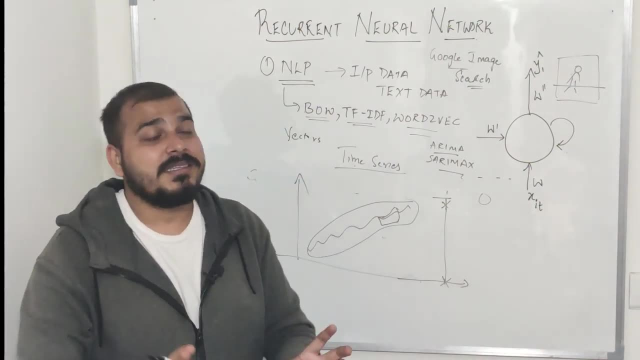 investing a whole lot of money for that. so recurrent neural network is definitely the most important. after what I'll say, that deep learning and recurrent neural network are most important in this particular techniques and I'll make sure that- and this just the part one, guys, I've just told you 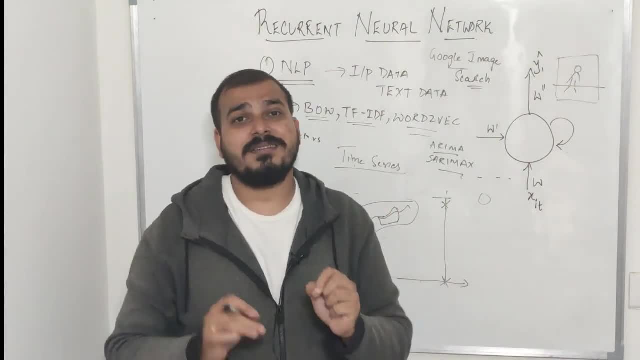 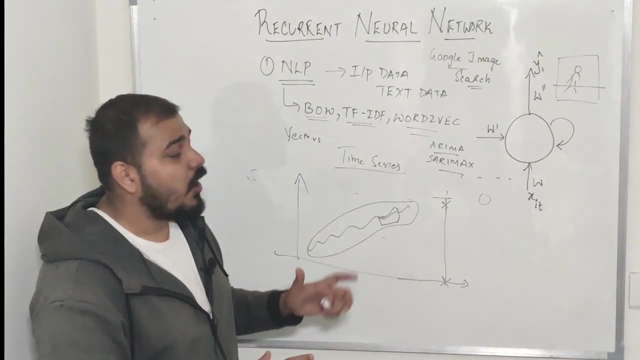 some of the application and this video is about why recurrent neural network and some of its application. in the next video, in the next part, I'll be discussing the maths behind it, and this maths will look awesome because I have explored this a lot and I'll make sure that I and I have literally done some.